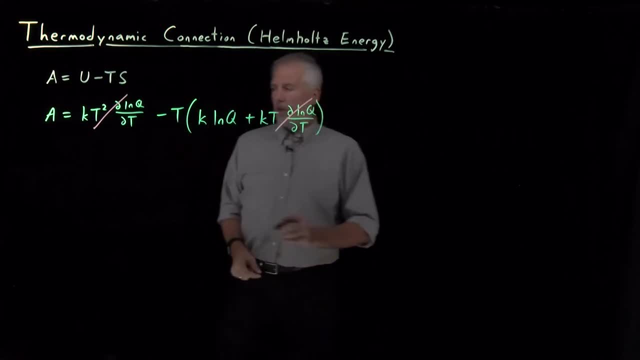 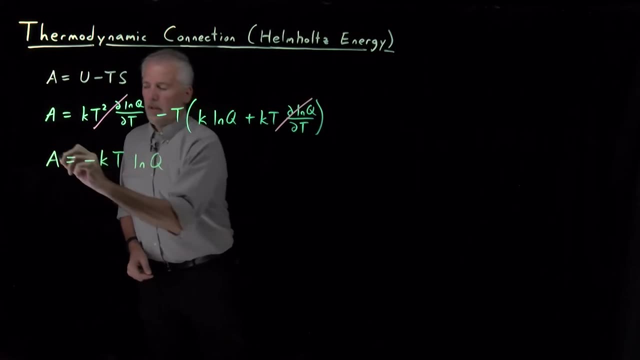 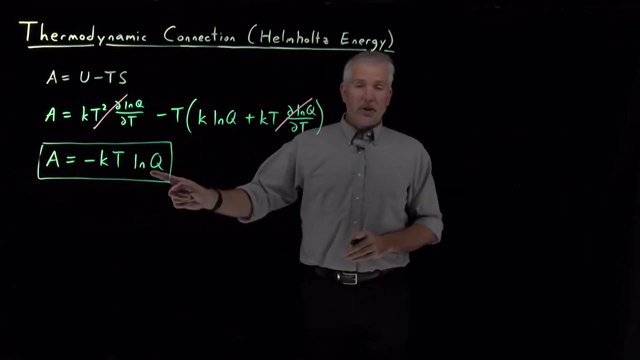 is this term negative kt times the log of q. So Helmholtz energy is minus kt log q. That's our Helmholtz. It's a thermodynamic connection formula for the Helmholtz energy. If we know what the partition function is, as we do, for example, for a particle in a. 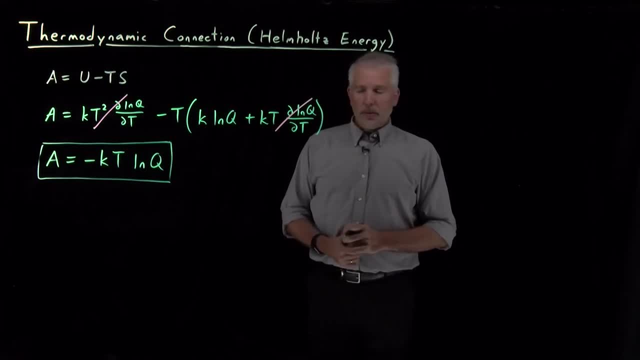 box or for an ideal gas or a rigid rotor or whatever. then we can use that expression for the partition function to obtain the Helmholtz energy of that particular system. So it's fairly striking how simple the form of this partition, this thermodynamic connection formula. 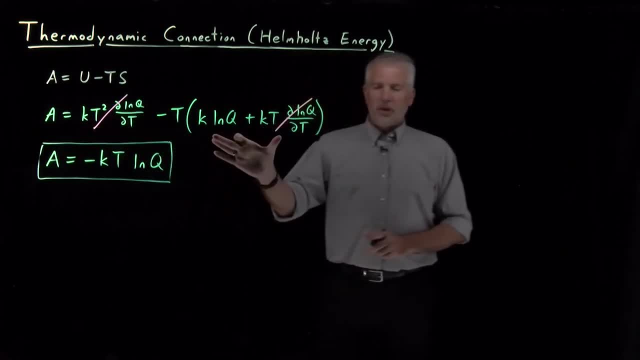 is. It's simpler than the one for the energy, simpler than the one for the entropy. In particular, it doesn't involve any derivatives of q or log q with respect to anything, as our other thermodynamic connection formulas have. The reason this expression is so simple as we've. 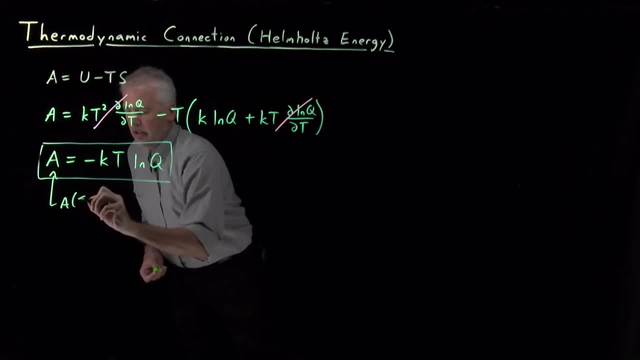 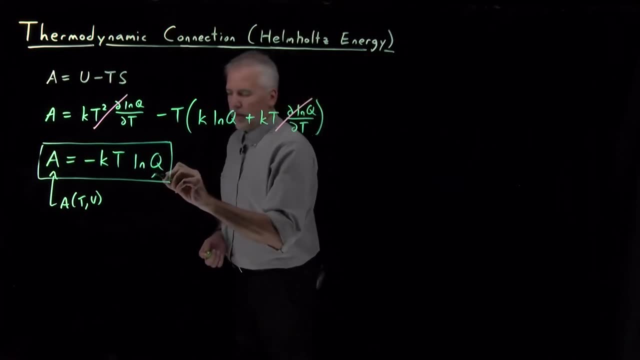 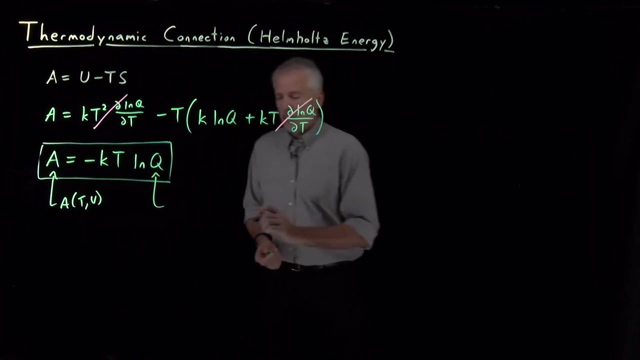 seen, the natural variables for the Helmholtz energy are the temperature and the volume. It turns out the natural variables- we haven't talked about it in this way, but the natural variables of the partition function q are also temperature and volume. What I mean by that? if we remember. 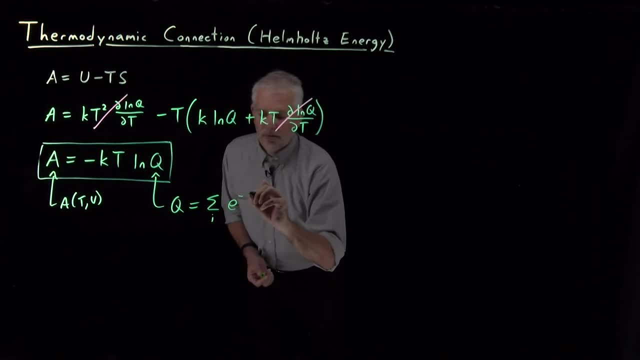 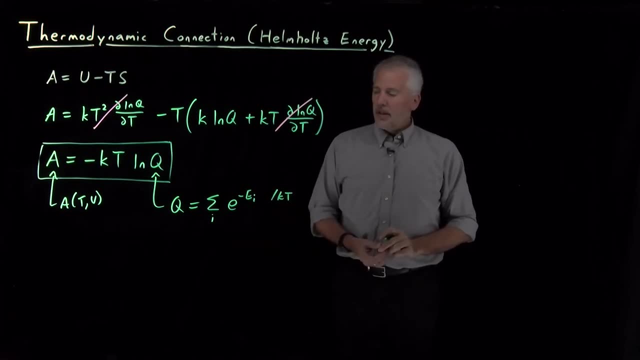 what the partition function is, that's the sum of Boltzmann factors, the sum of e to the minus energy divided by kt. summed over all the states, the system can have Energies, the energy, if we think about a system like a particle in a box, for example. 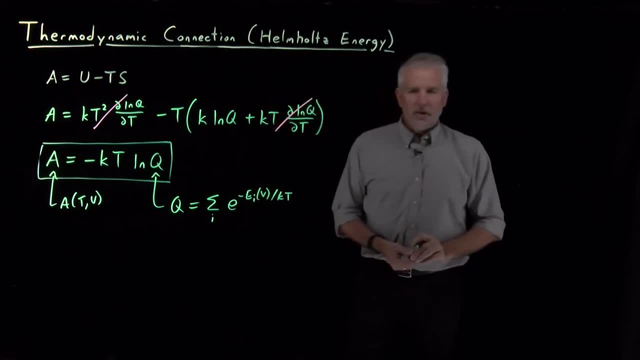 the energies will depend on the volume. If I change the volume of the system- any quantum mechanical system confined to some volume- that volume affects the energies. If I change the volume, it affects the energy levels. The energies depend on the volume, The temperature. 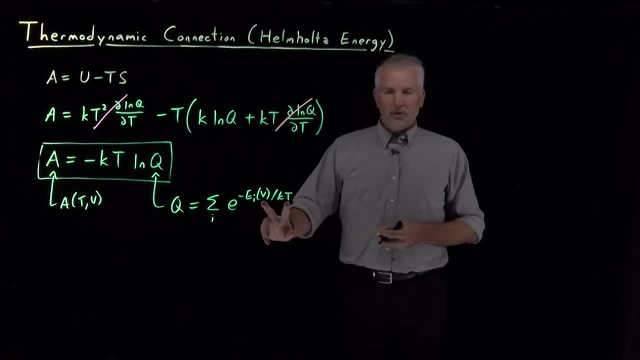 also shows up in this expression. The most natural thermodynamic variable dependence of the partition function is on these two variables, V and t. Since q is a natural function of V and t, a is also a natural function of V and t. that means the relationship between: 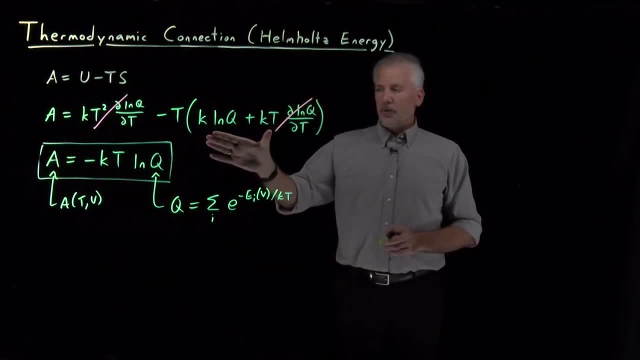 them is relatively simple. The thermodynamic connection formulas for these other quantities like entropy or log kt are fairly simple If we change the weights of t and q and a or internal energy are not quite as simple because it involves changing from a function of T and V.